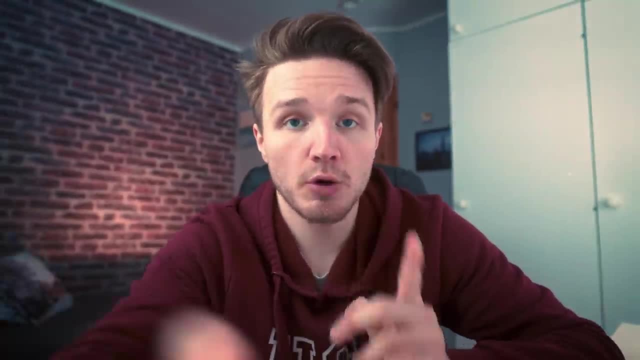 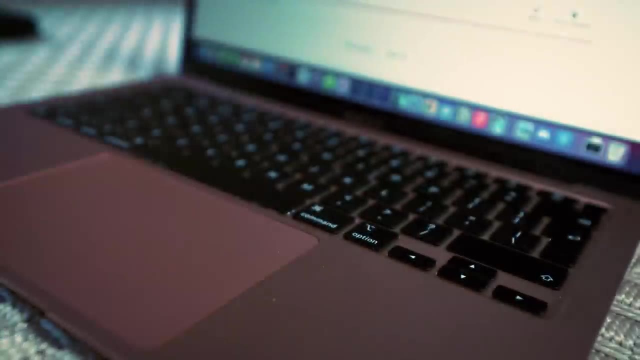 that math wouldn't be useful for programming. I understand both arguments, So in this video I'm going to do my best to reconcile them, And my conclusion will be that, while in most applications of programming, you're probably not going to be using all that much complicated math, 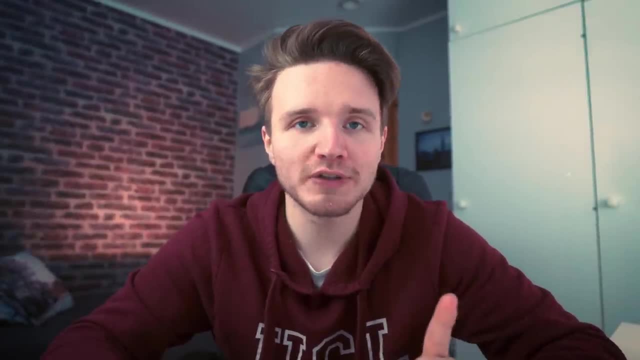 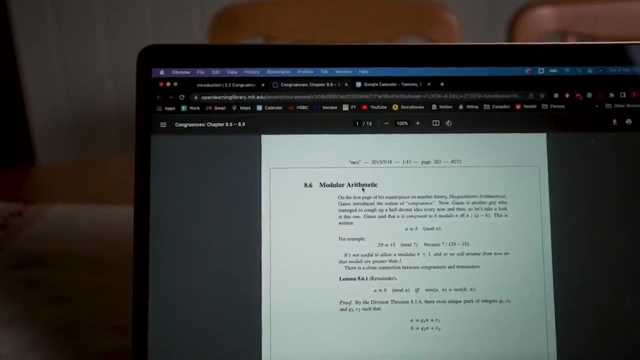 you should probably still learn it. And what's more important than that conclusion is how I get there, And that's what I'm going to try to explain in this video, And at the end, I also give you my recommendation for the best free resource to learn all the math you'll ever need for. 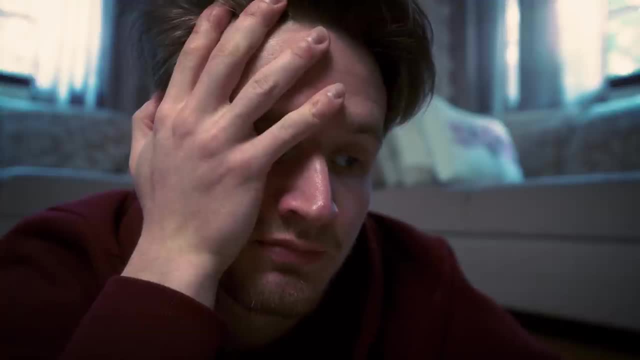 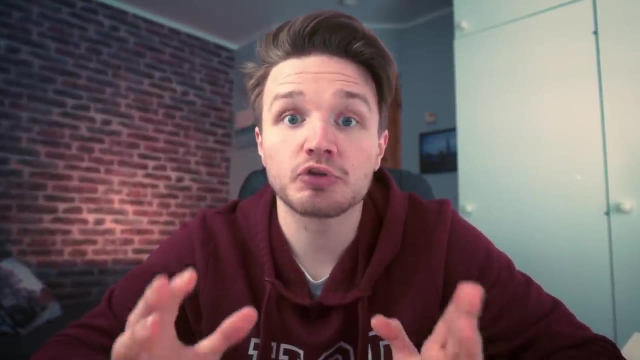 computer science. So definitely stick around till the end for that. So the real answer of whether you need math for programming is: it depends, which I know I know is the most boring, the most annoying, the most frustrating answer ever. So let me just explain that. The question of whether you 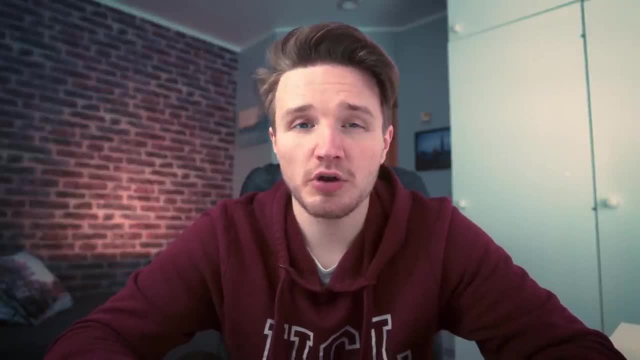 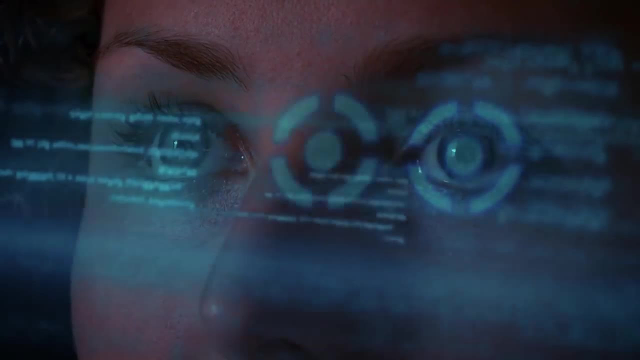 need math, for programming doesn't really make sense without some context. It all depends on what you want to create, which area of programming you're getting into, what your future goals are- all these kinds of things, Sure, if all you want to do is make a simple website using HTML CSS. 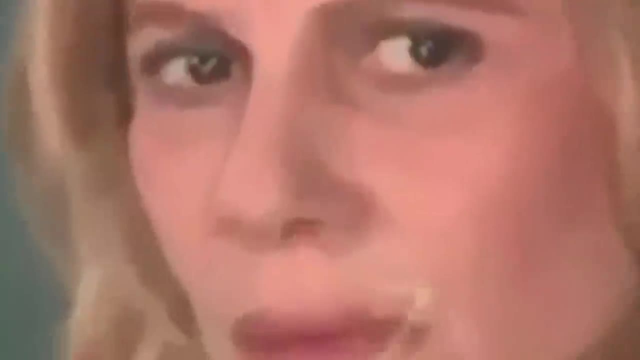 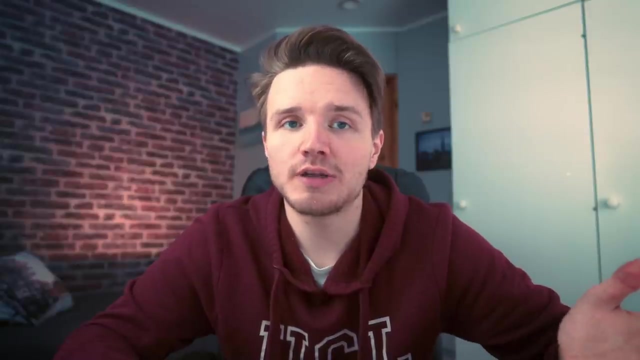 and JavaScript, then sure you're not going to need to know how to multiply matrices together or how to find a topological sort of a finite directed acyclic graph. So if that's all you want to do, then there you go. You're probably not going to need any math. Thanks for watching, But here's. 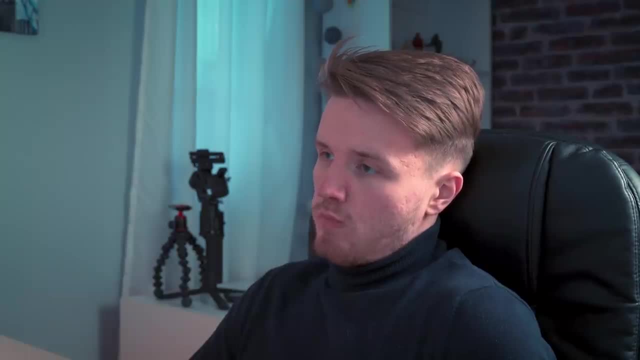 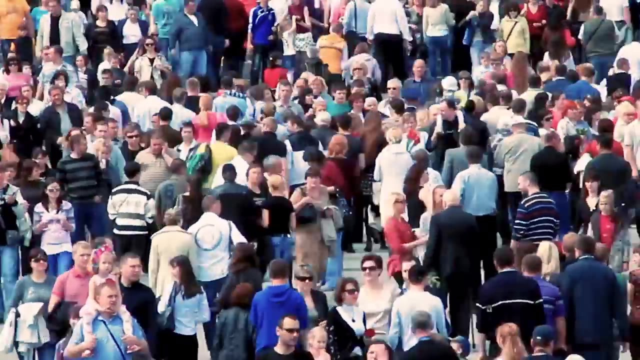 why you should still learn the math. If all you know how to do are those simple tasks, then you really aren't providing that much value, Because if something is easy to learn, then there's going to be an abundance of people who know how to do it. So, in general, you should try to become the 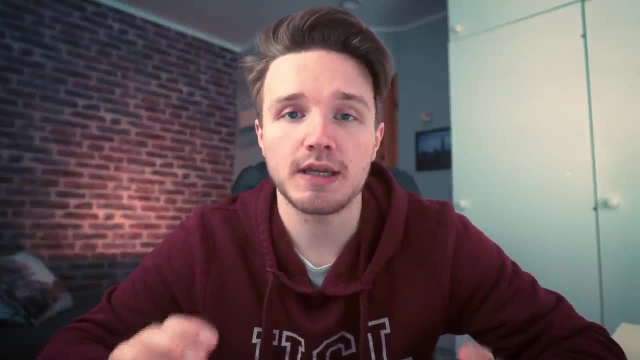 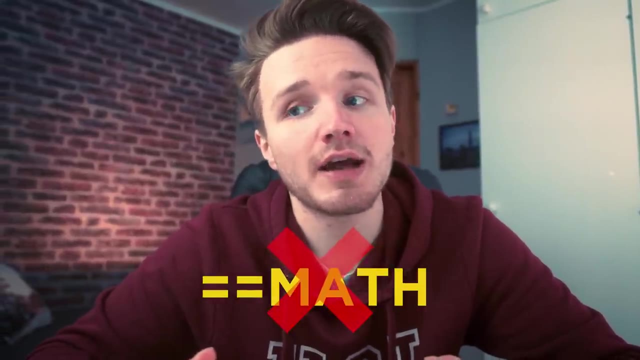 most amount of knowledge that you can possibly get, And that's where the math really comes in. It's very easy to make the argument that most people who get started in programming start in web development, and in web development you don't really need that much math. So therefore, you just 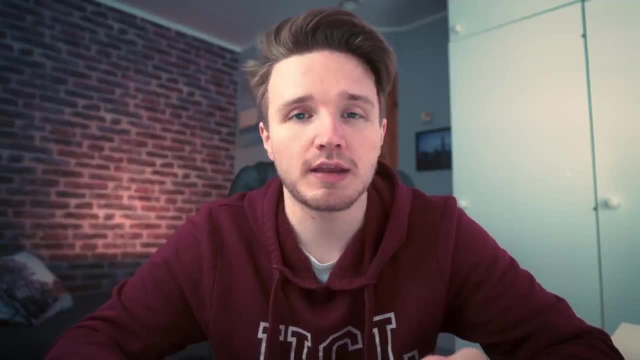 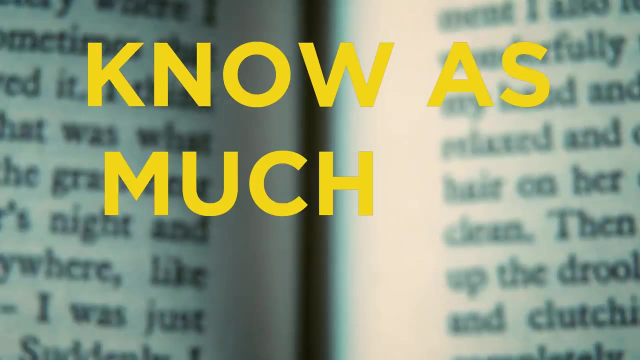 don't need to learn it. But I think that's a misguided style of thinking And if you take this attitude, it can lead to problems down the line. Just in general, I always think that you should err on the side of trying to know as much as possible- Knowledge, Because knowing more can. 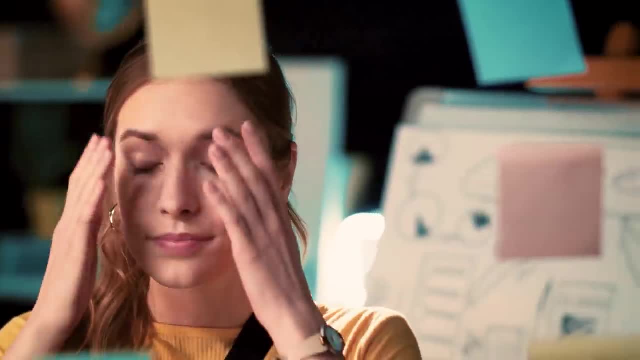 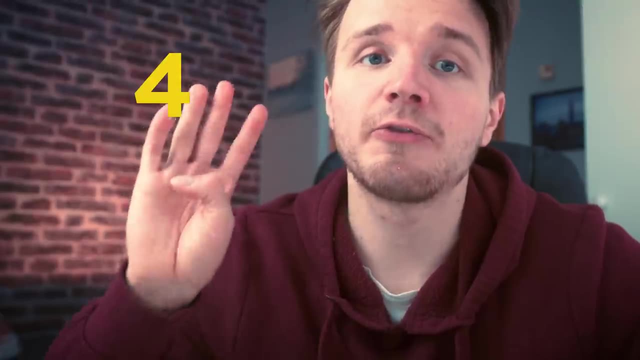 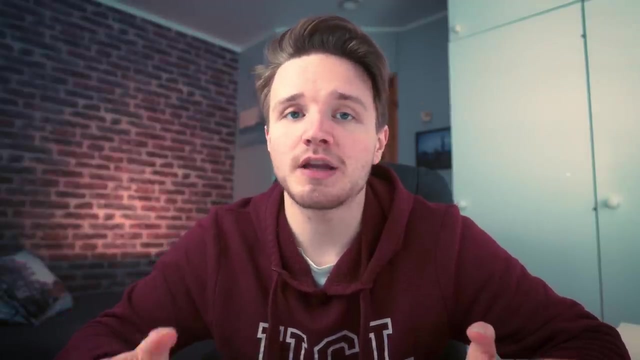 never be harmful, whereas not knowing something or not fully understanding the fundamentals of something can come back to bite you later on. However, if that general argument alone doesn't convince you, here are four specific, concrete reasons why you should absolutely learn the math required for computer science, even if you don't want to become like a theoretical computer. 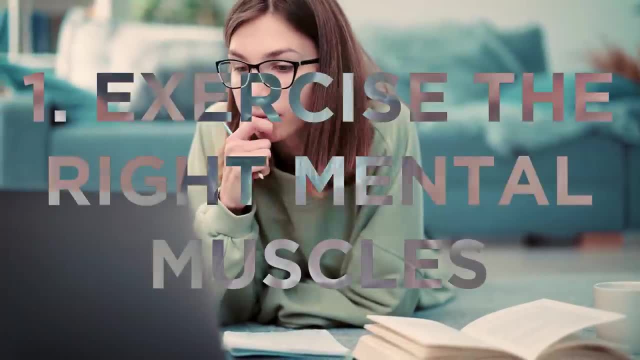 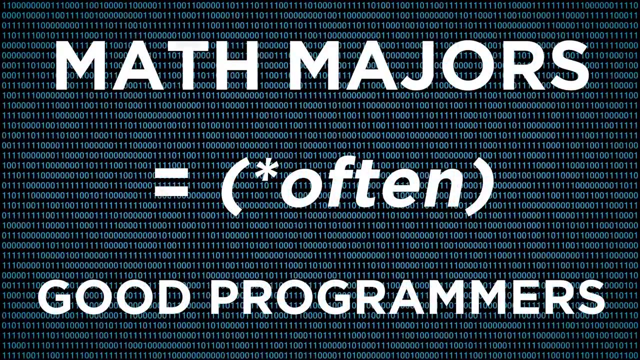 scientist or something like that. First reason is that math exercises the right muscles, And what I mean by that specifically is that I've heard many people in the industry say that math majors usually rank among the best in coding boot camps and that kind of stuff And they generally make very good. 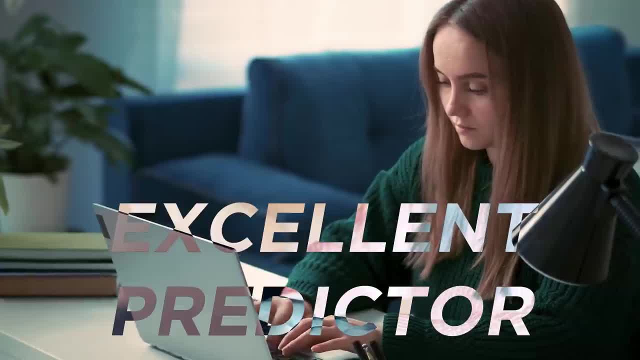 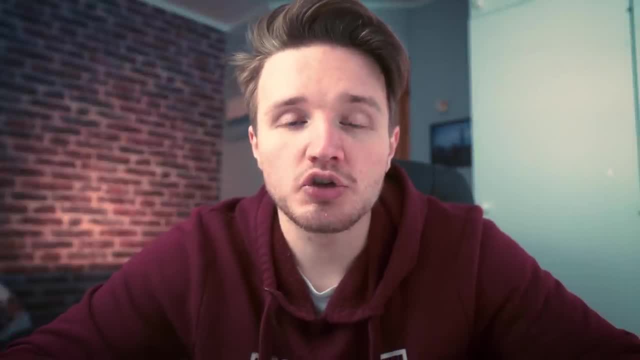 math, And I think that's a good thing. And I think that's a good thing, And I think that's a good thing And crucially this is: this is not because you would specifically be using that math in your job, but rather because thinking about math problems and thinking about programming problems largely 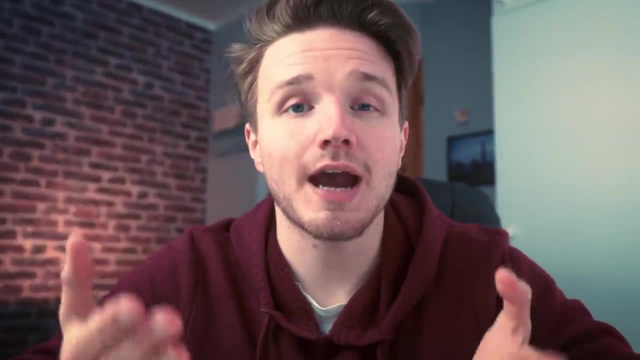 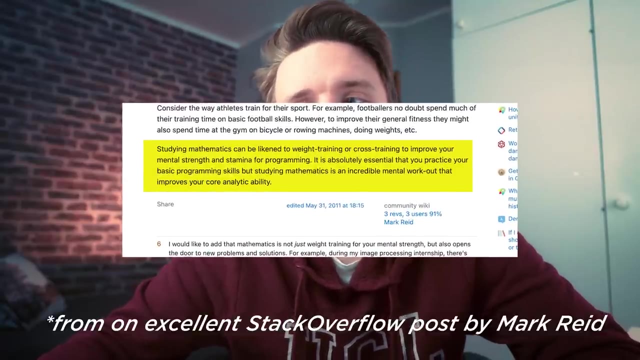 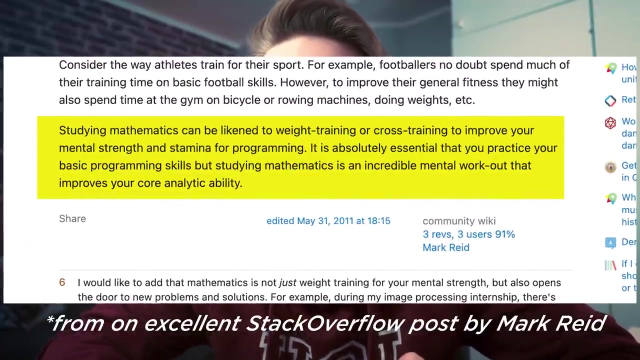 uses the same kinds of mental muscles or the same kind of reasoning. Studying mathematics can be likened to weight training or cross training to improve your mental strength and stamina. for programming, It is absolutely essential that you practice your basic programming skills and programming skills, But studying mathematics is an incredible mental workout that improves your 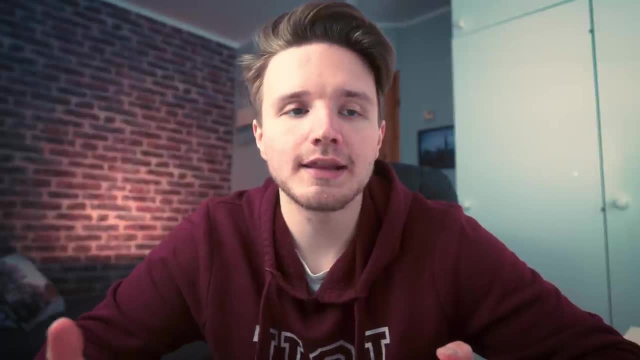 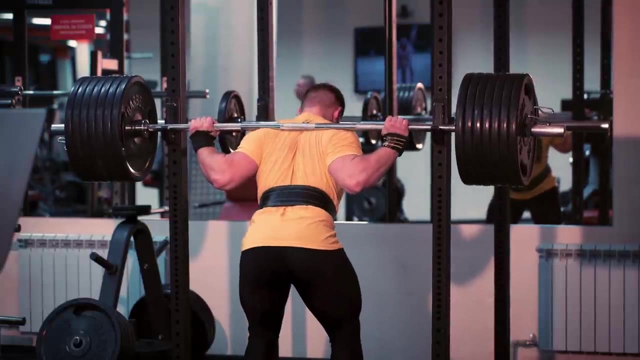 core analytic ability. So you can think of an athlete who wants to do well in football, for example. doing squats at the gym is not directly what they need to be doing as a footballer, but it exercises the right muscles to build their leg muscles, which will then, in turn, be useful when 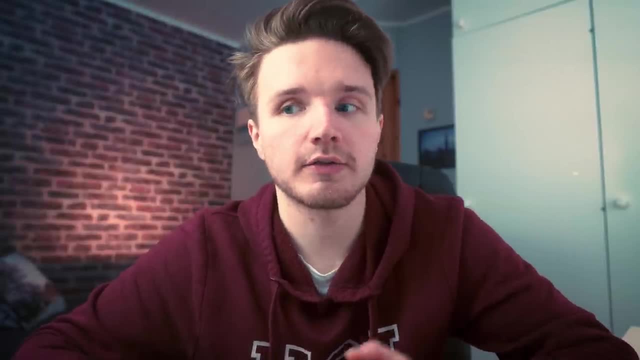 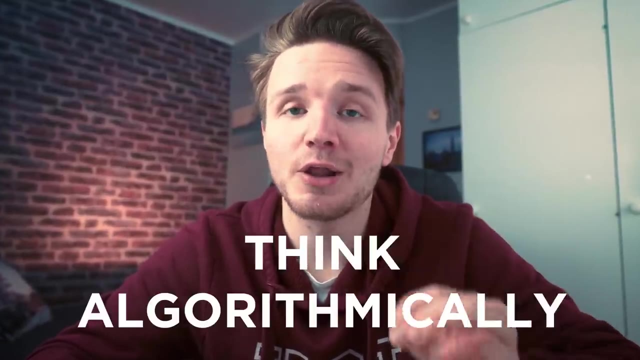 they're playing football because it will allow them to run faster, and that kind of stuff. So otherwise, there's a strong correlation between understanding mathematics and being good at programming, That is, being able to think algorithmically. Reason number two is that you develop a more 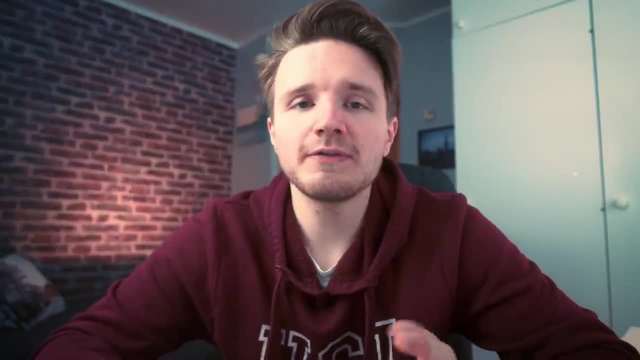 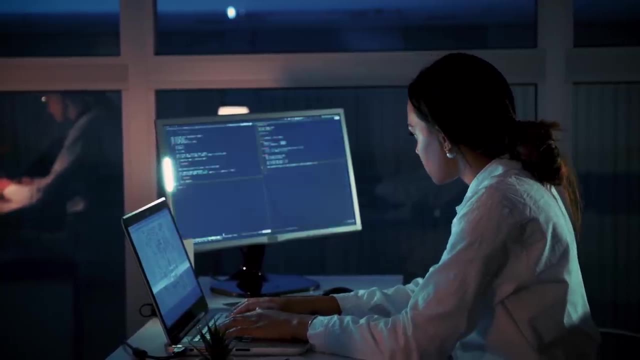 fundamental understanding of programming concepts. Even if 99% of the time you're not using that much math in programming, there's still that 1% of cases where you really need it and where understanding it is going to make you a better programmer. Programming is essentially just a 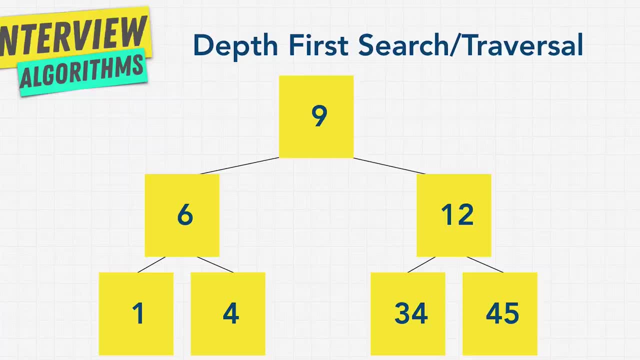 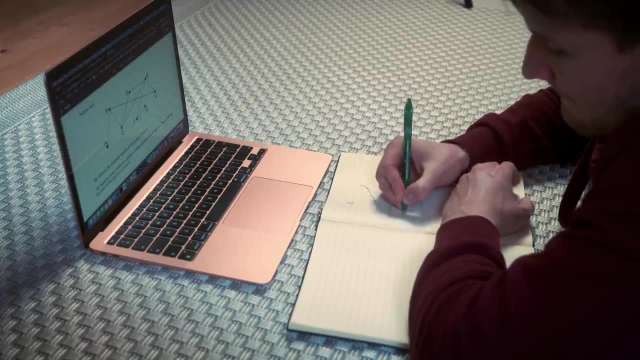 subset of math. Algorithms are just a set of instructions based on mathematical logic, and data structures are similar to just found in math too. Even with my limited experience, I've already seen many cases where the fact that I studied math for computer science before going into studying 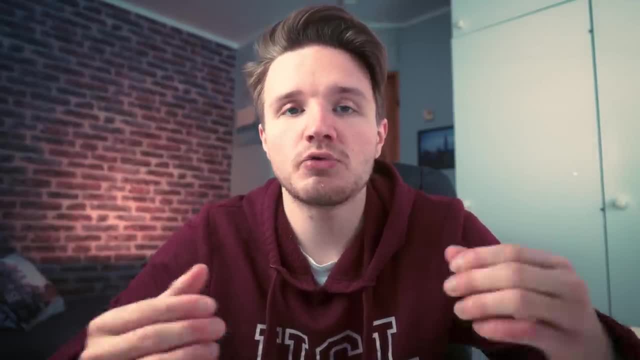 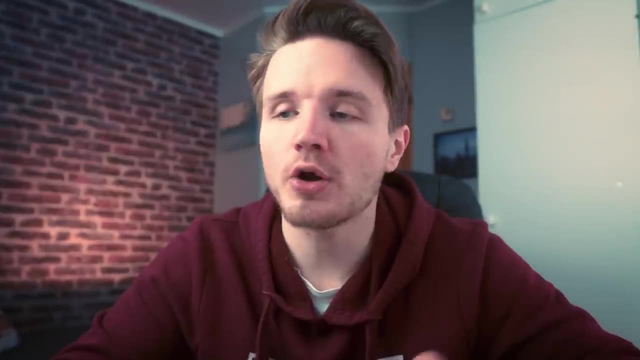 programming and studying data structures more helped because I have a way more fundamental understanding of where all these concepts actually come from which I can actually understanding, rather than just trying to memorize like, okay, you use an array here, you use a graph in this. 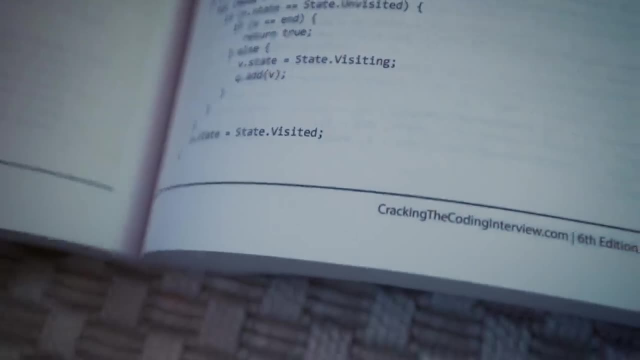 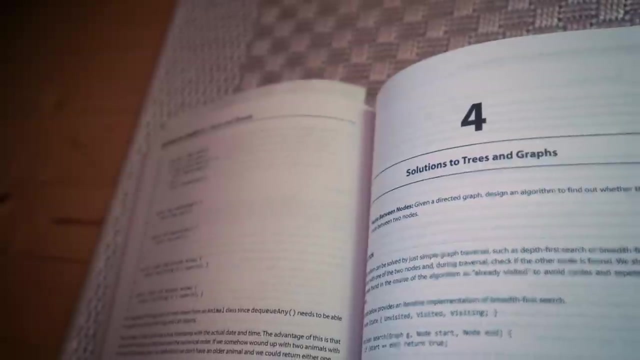 kind of situation. I don't need to memorize anything, because I can just understand why those things are. It makes sense to me because I understand graph theory and these kinds of things already, Even topics that you wouldn't think are that useful, like understanding what your. 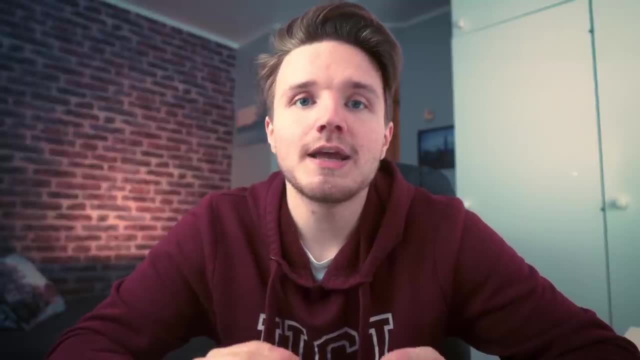 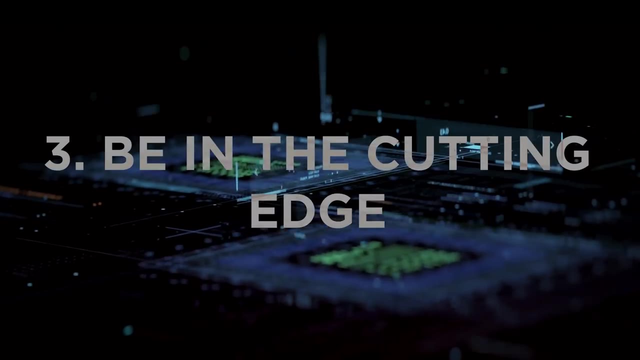 algorithm is, and then you can just use that to figure out what the actual algorithm is. I've also been using the word modular arithmetic because I've already been finding many practical applications for the modular operator in a lot of programming languages. So reason number three: 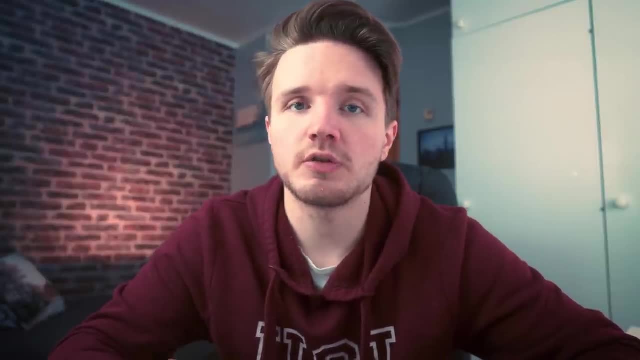 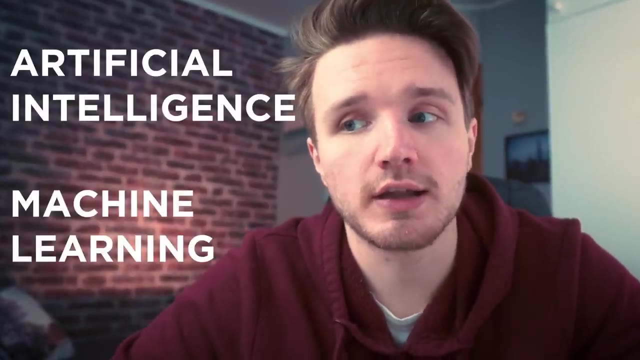 is if you want to be at the cutting edge. So you know from my previous videos that software engineering is an extremely high demand industry, but want to be in an industry that's even more in demand than software engineering, you should look into artificial intelligence and machine learning. 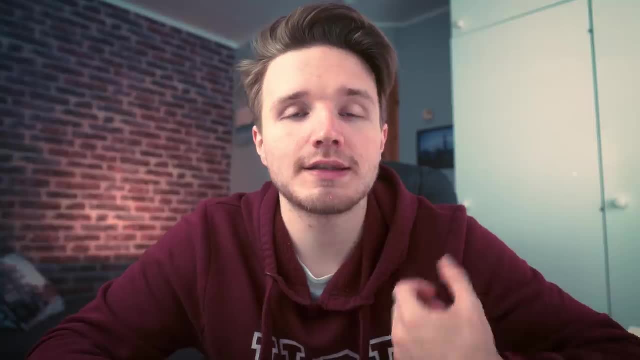 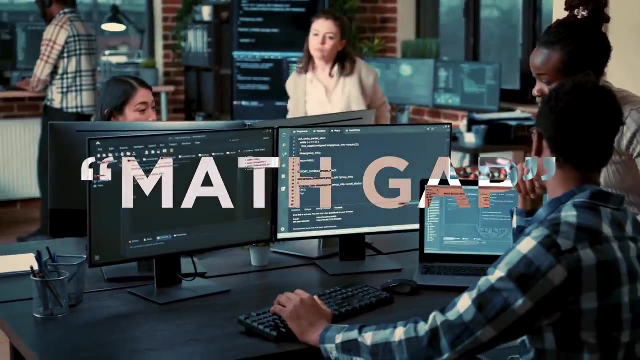 These are subfields of computer science that draw on a lot of math, a lot of probability and statistics and a lot of data. So if you want to be at the cutting edge of the technology industry, it's happening. In fact, people often talk about a math gap, with many software engineers who want 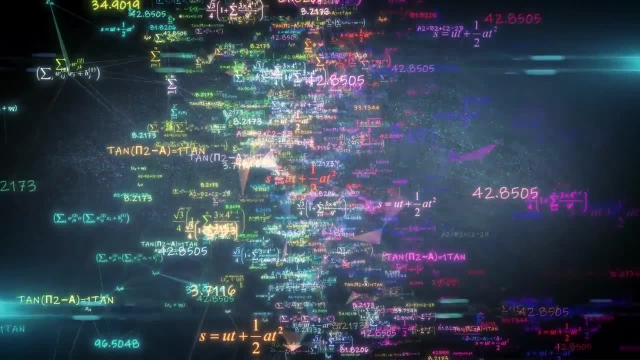 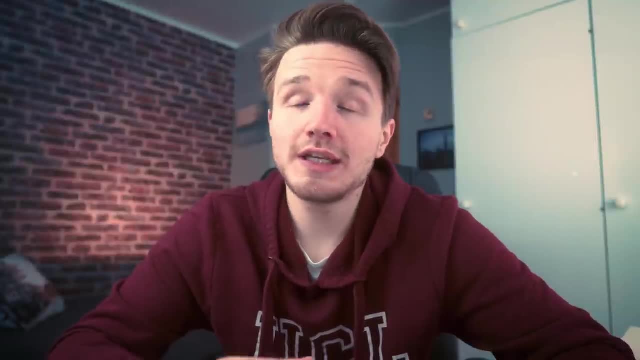 to transfer into one of these fields. And even if you don't want to go into these subfields, it's still just a general good strategy to know all the fundamentals, to understand the fundamental math behind computer science. So then, in the future, if you do need to adapt, if you do want, 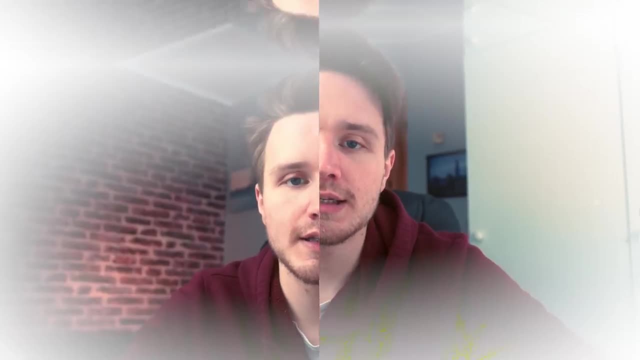 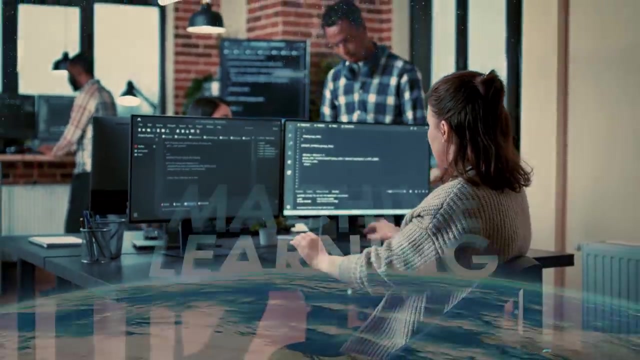 to go into something else. you can do it much easier when you already have that fundamental understanding. The technology industry is, by its nature, evolving extremely fast. You never know what's going to happen. in 10 years, A lot of the basic programming stuff have been automated by. 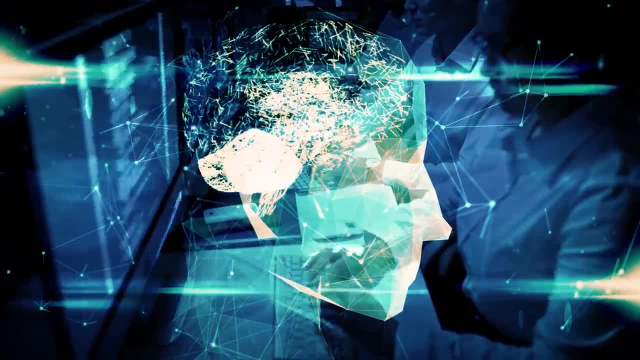 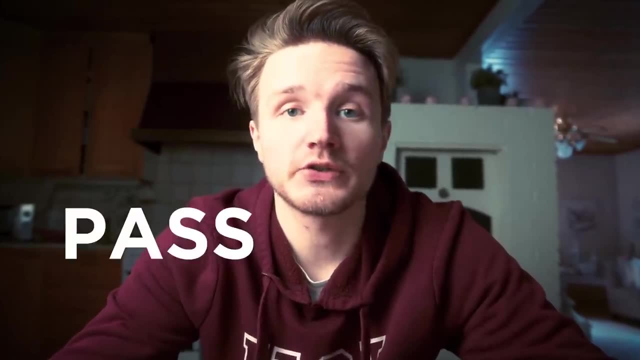 AI algorithms, for example. So you never know if, for your own job security, you might have to transfer into one of these fields in the future. And last but definitely not least, you should learn math, because it will actually help you pass coding interviews. This sort of ties into the 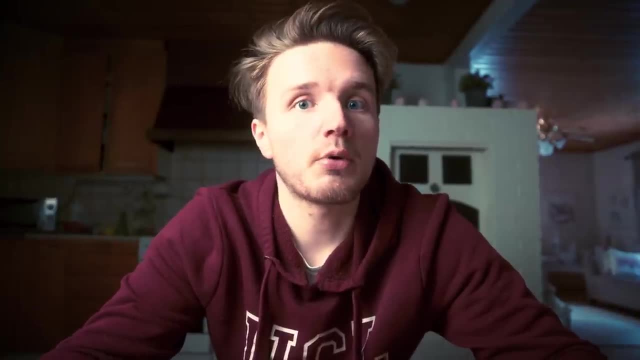 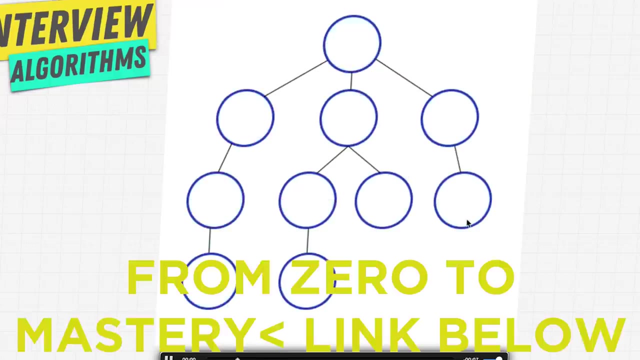 previous points, but I wanted to add this in there because, let's face it, this is probably the point that's going to convince most people. Knowing math will help you pass interviews because it will help you understand those underlying concepts that a lot of tech interviews do. 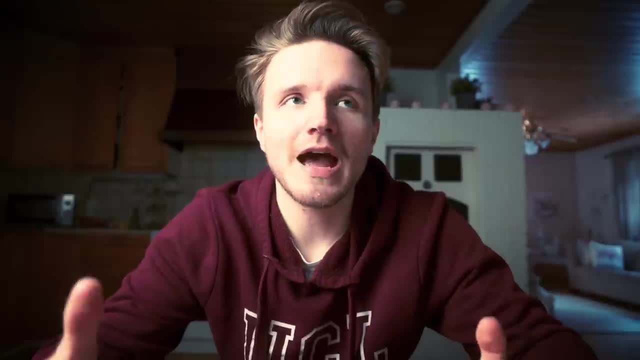 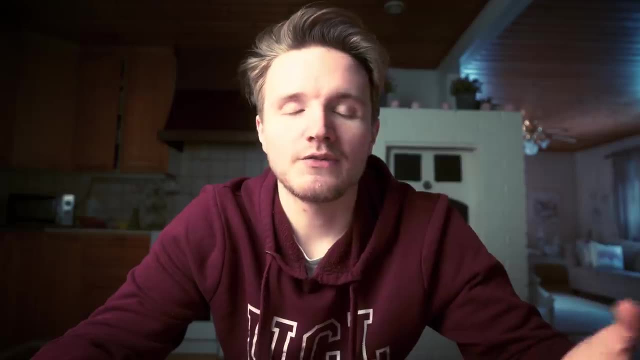 Test for, specifically, data structures and algorithms. I cannot believe how many people there are who are studying for coding interviews by just memorizing a bunch of leetcode questions, Like, if you have an interview tomorrow, you're memorizing some leetcode questions and then 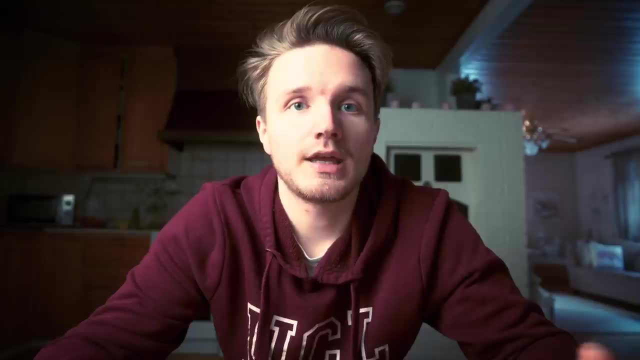 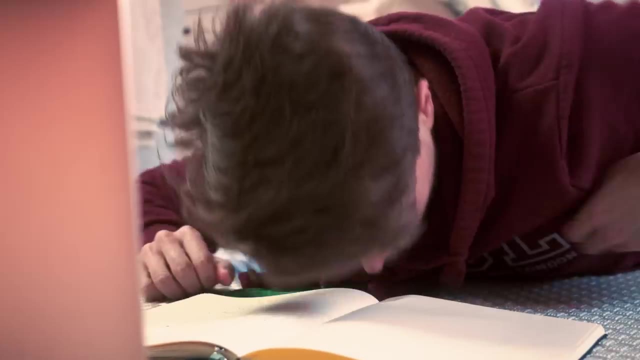 hoping you get lucky- that those are the questions that you're then tested on. It can't work. But let's say you study like that for a coding interview and then in two months you have another interview. You'd have to do everything all over again And it's generally much harder. 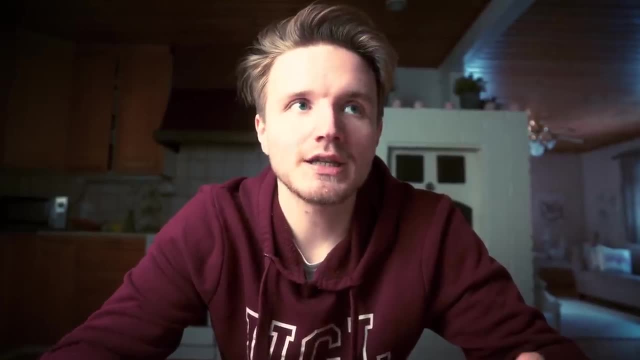 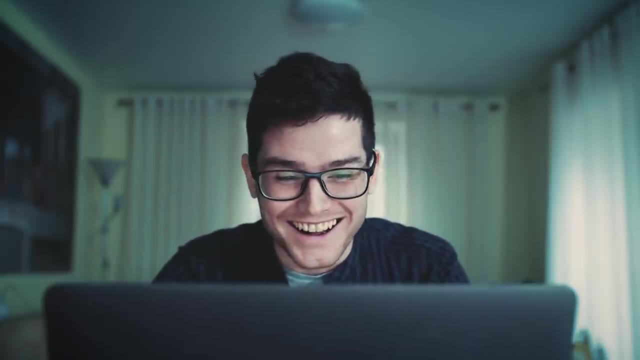 to memorize stuff that you have no underlying understanding of than just spending your time upfront to properly understand the theory and the fundamentals behind these concepts. So by properly understanding and internalizing these concepts, you can then just not have to worry about any interview really, because you'll have the underlying understanding that you can. 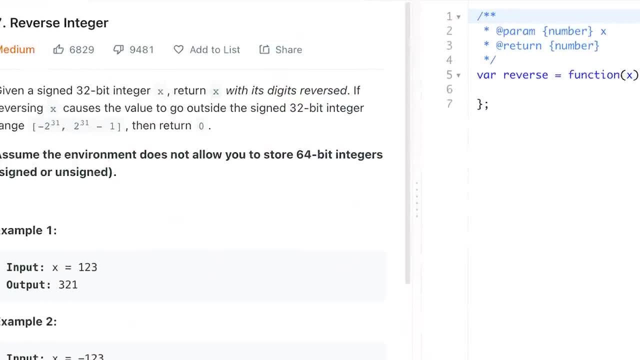 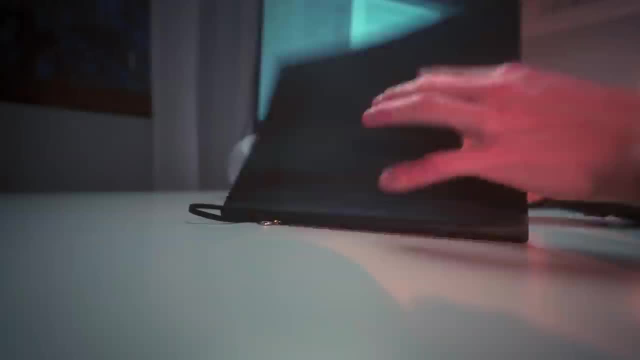 then apply to any problems. After all all the problems in leetcode and interviews. they are based on data structures and algorithms and a lot of the computer science concepts. Having done the math beforehand just helped me so much in being able to visualize and really 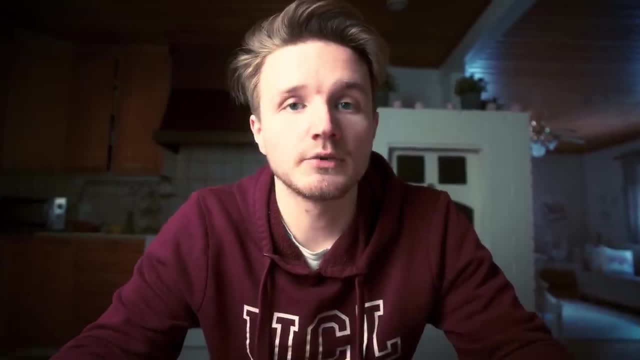 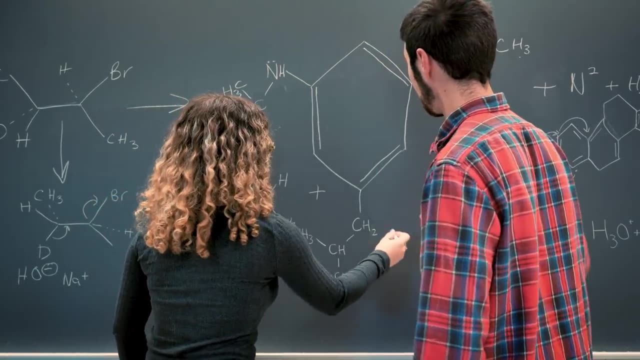 understand what's going on with a lot of these things. All because I took the time to study the math. So, as a conclusion, you shouldn't be deterred by the math. Math is hard, but it's also the most beautiful and pure manifestation of logic and problem-solving. 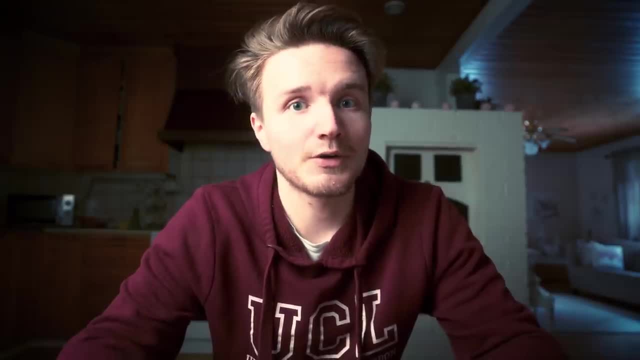 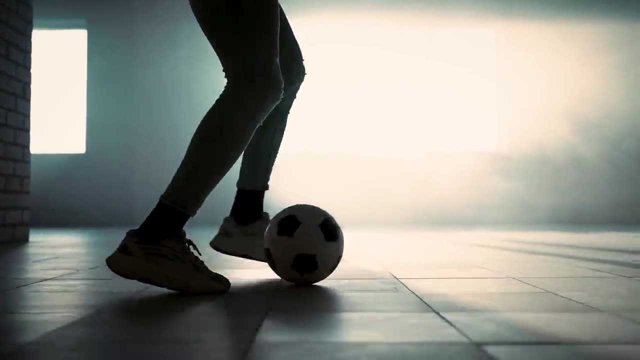 Any valuable skill is going to be hard to learn, And math is definitely no exception. People seem to have a bigger initial aversion to it than most other skills. After all, getting good at football, for example, is also very hard, But because it's something that I don't know like looks easier. 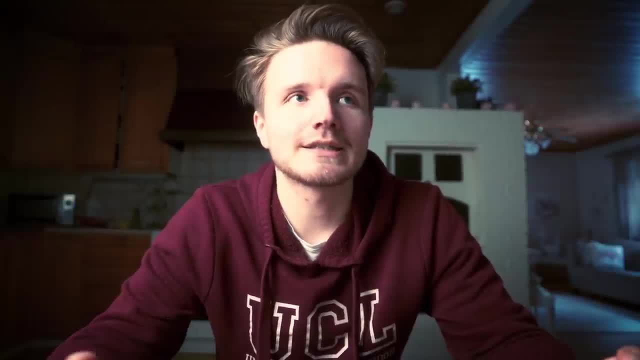 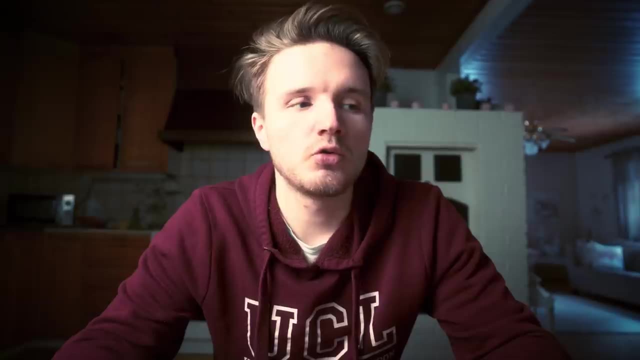 and it's not like abstract. in the same way as math is, people aren't as scared of trying to be good at football. So I challenge you, if you want to be good at football, to do it. So I challenge you to embrace the challenge. with math, You should become the type of person who wants to master. 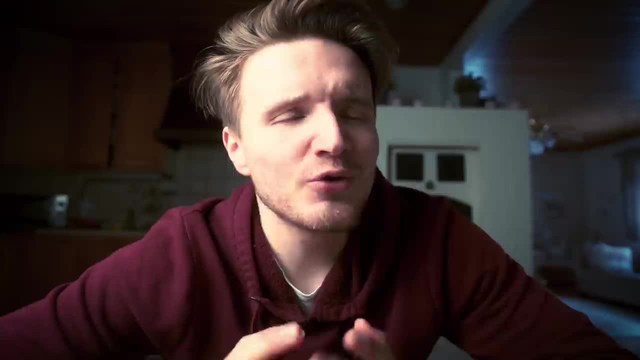 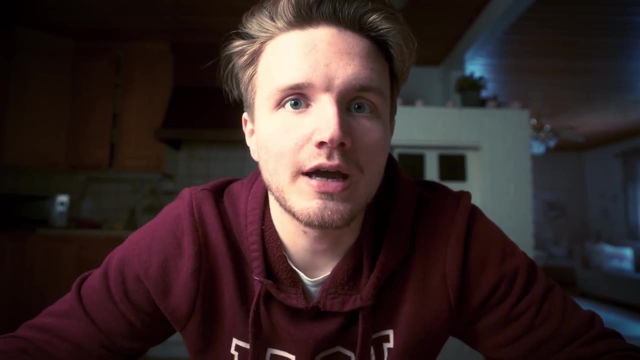 these skills and who wants to master hard skills in general. How cool would it be if you could be the person who understands math and who's really good at it, when most people aren't able to do that. And you can do it if you just put in the work to learn it. So I also challenge you to adopt 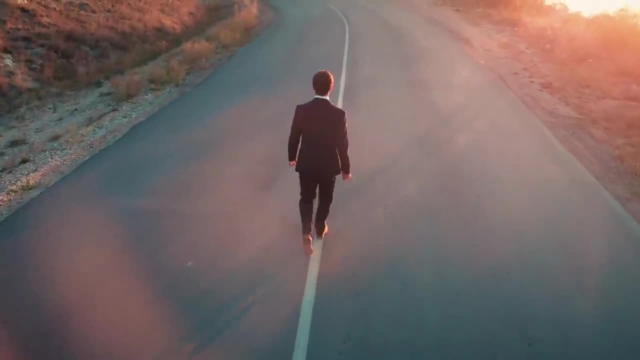 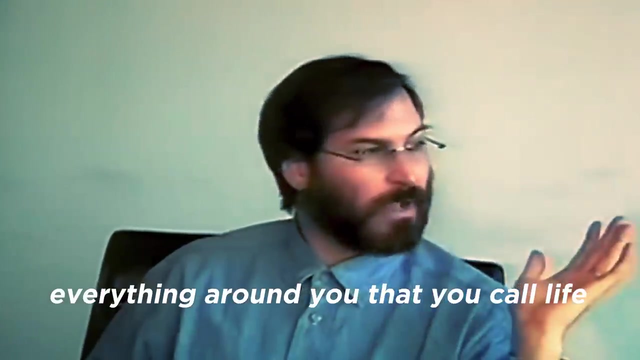 a growth mindset, which means if someone else can do it, you can do it too. if you just put in the work, Life can be much broader once you discover one simple fact, and that is everything around you that you call life was made up by people that were no smarter. 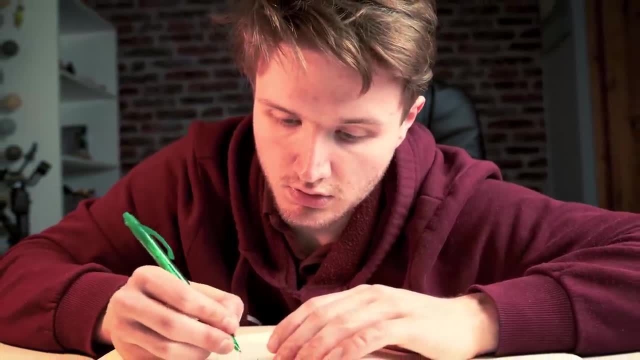 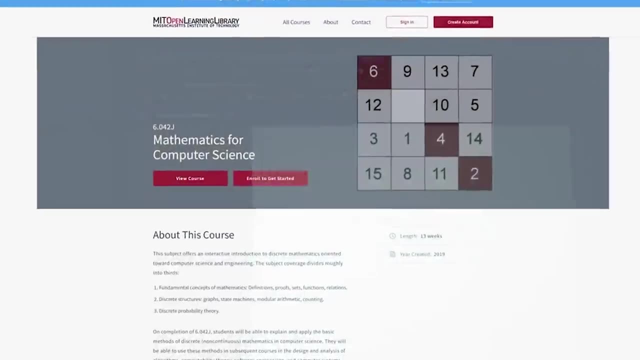 than you. So, in terms of a specific resource to get started learning math and computer science, the one that I did was MIT's free course called Mathematics for Computer Science. There's also a version of this course on YouTube, which just has a lot of video lectures, But I do actually. 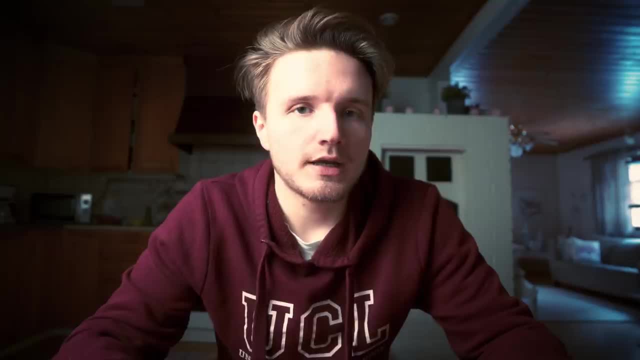 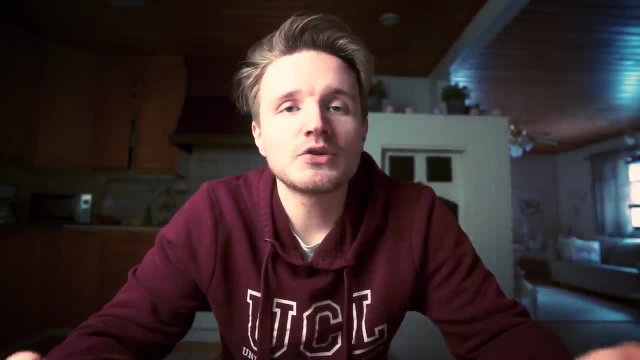 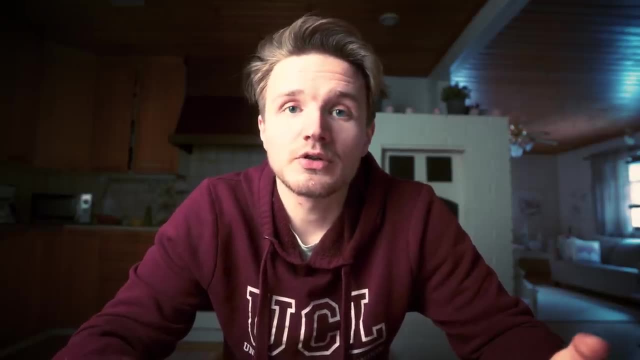 coding computer science you can just do on the internet, And this is essentially what I am doing. I'm teaching myself a whole curriculum on computer science using free online materials, And if you want to learn how I'm doing that, if you want to do the same, you should definitely. 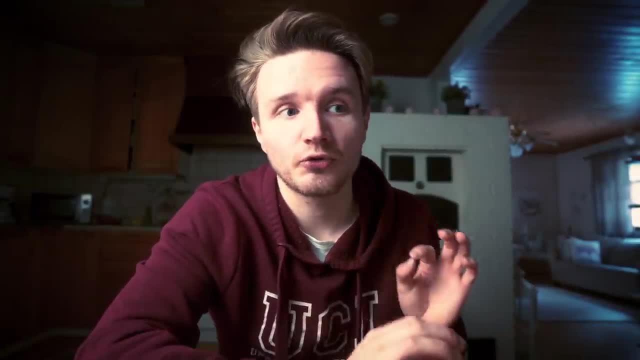 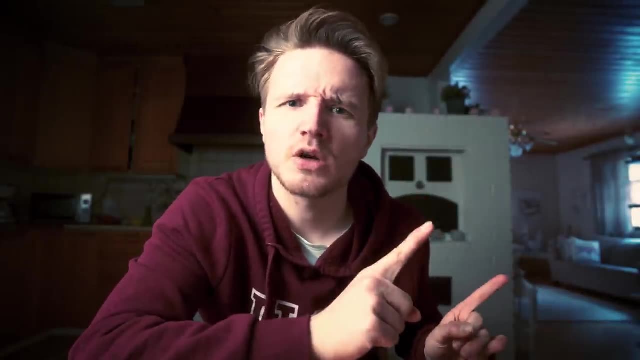 check out this video next, And I include a free notion template for you to follow along and study essentially a full computer science degree online without even going to any proper university. So yeah, definitely go watch this video next.